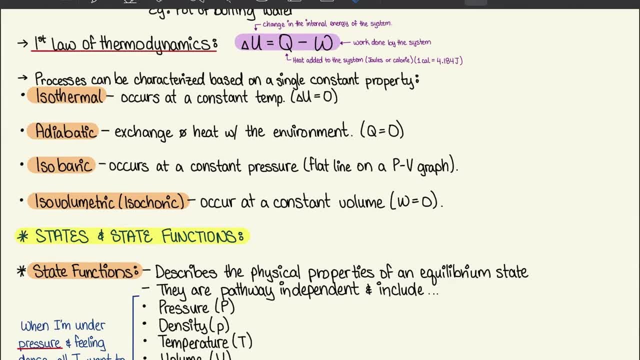 system. So the processes can be characterized based on a single constant property. So we have isothermal that occurs at a constant temperature and that's where our delta U is equal to 0. So the internal change of energy in the system is zero, So there's no change happening and that would be your isothermal. 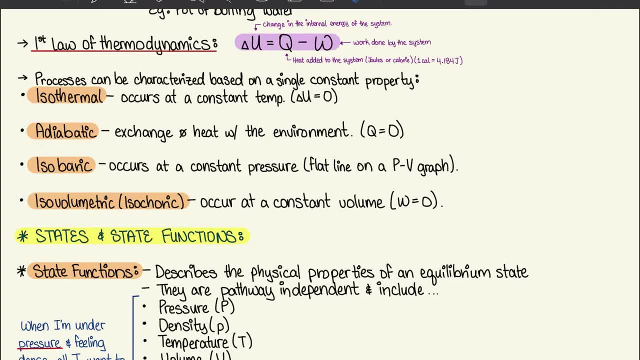 For adiabatic. it exchanges no heat with the environment, So your Q is equal to zero And Isovolumetric occurs at a constant pressure. so on a pressure-volume graph you'll just see a flat horizontal line And isovolumetric occurs at a constant volume. so the work is equal to zero in this scenario. 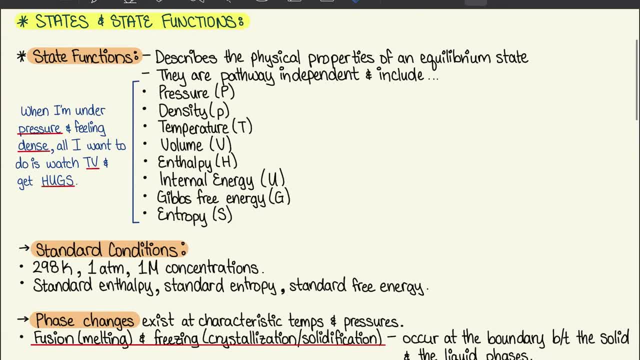 Moving on to 7.2,, we have states and state functions. So state functions describe the physical properties of an equilibrium state and they are pathway independent and include pressure, density, temperature, volume, enthalpy, internal energy, Gibbs, free energy and entropy. 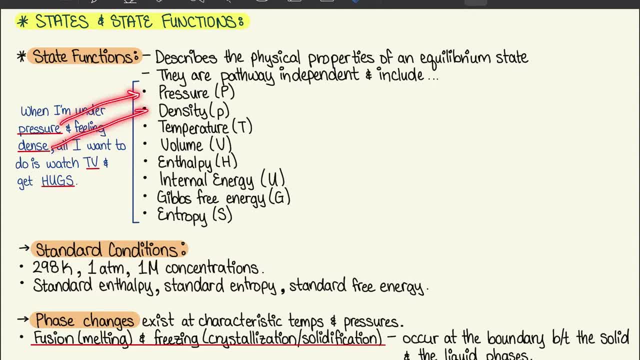 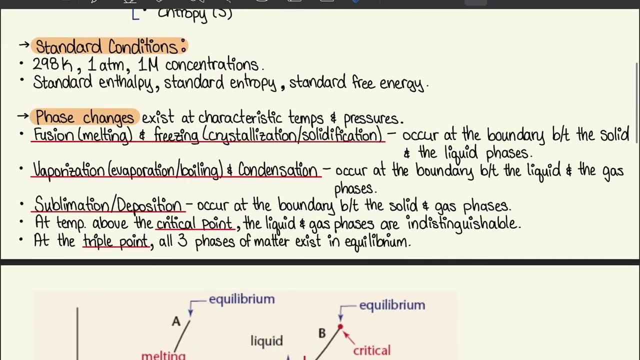 The mnemonic for this is when I'm under pressure and feeling dense- and dense would be the small p- all I want to do is watch TV and get hugs, So hopefully that helps. For standard conditions we have 298 Kelvin, one atmospheric pressure and one molarity concentration. 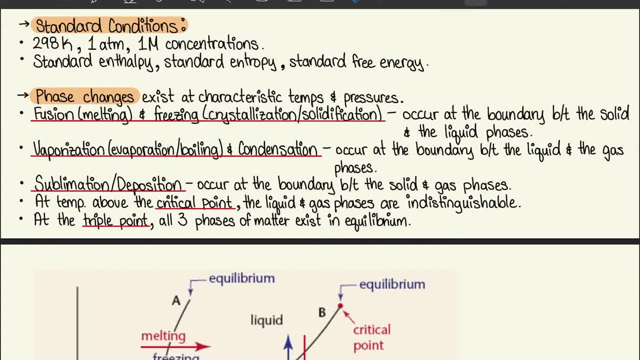 It's standard enthalpy, standard entropy and standard free energy And we have phase changes that exist at characteristic temps and pressures. So fusion, which is melting, and freezing, which is crystallization and solidification, occur at the boundary between the solid and liquid phase. 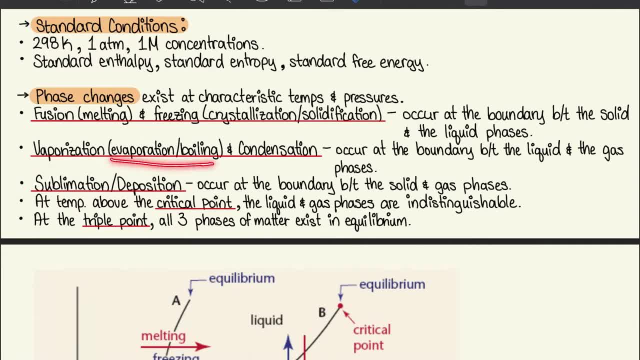 Whereas vaporization, which is evaporization or boiling, and condensation, which occur at the boundary between the liquid and the gas phase, We have sublimation, or deposition, that occur at the boundary between the solid and gas phases And at temperatures above the critical point. the liquid and gas phase are indistinguishable. 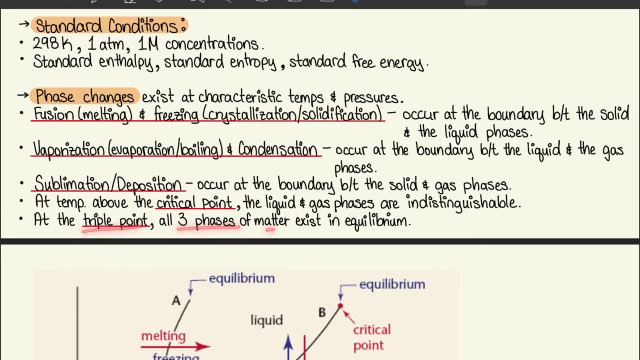 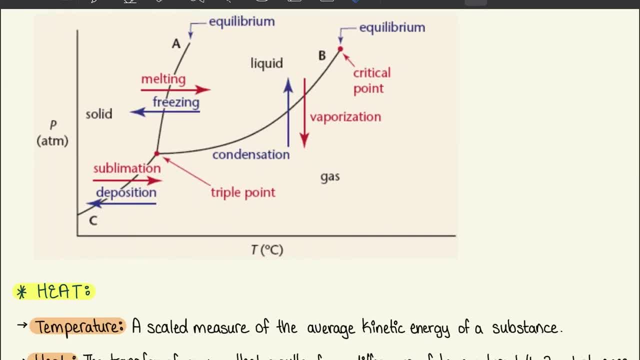 And at the triple phase, all three phases of matter exist in equilibrium And I have a graph. I have a graph down here below to show that exact thing. So pause the video and have a look at this graph and what we were talking about before and see if you can make those connections. 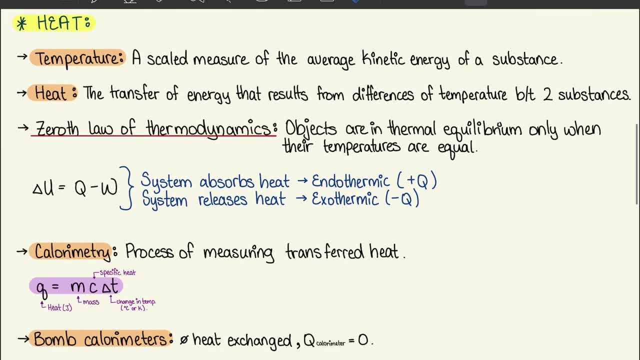 Moving on to 7.3, we're going to talk about heat. So the temperature is a scaled measure of the average kinetic energy of a substance, whereas heat is the transfer of energy that results from the differences of temperatures between the two substances. 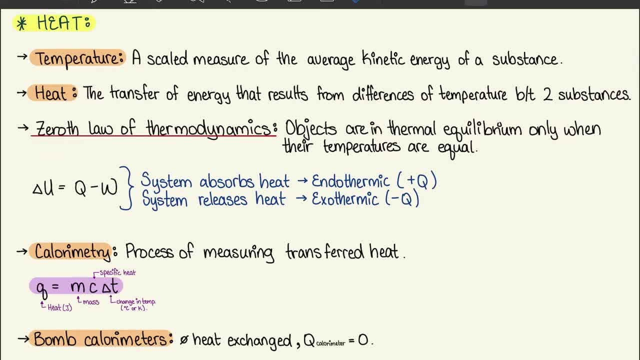 Here we have the zeroth law of thermodynamics, where objects are in thermal equilibrium only when their temperatures are equal. So we have the same equation from the first law that we talked about before. So it's delta U is equal to Q minus W. 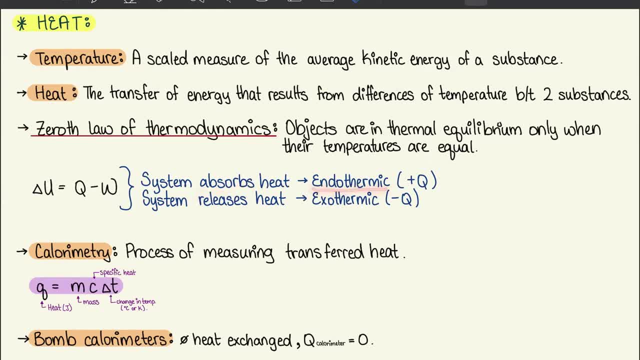 And when a system absorbs heat, it becomes endothermic, so we have a positive Q value. If the system is releasing heat, it's exothermic and we have a negative Q value. So, moving on, we have a calorimetry. 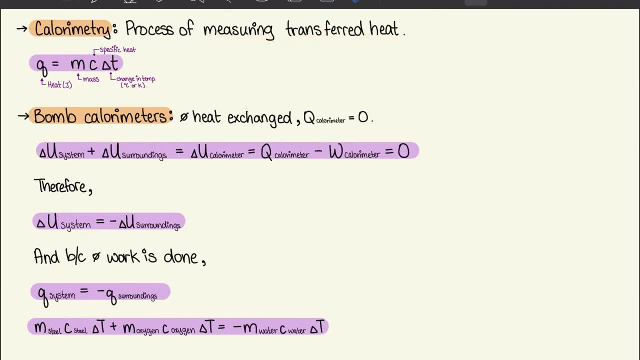 And that's the process of measuring transferred heat. And here we have the equation where Q is equal to MC delta T. So the way I like to remember this is: MCat is cubed with a Q, So the Q refers to the heat which is measured in joules. 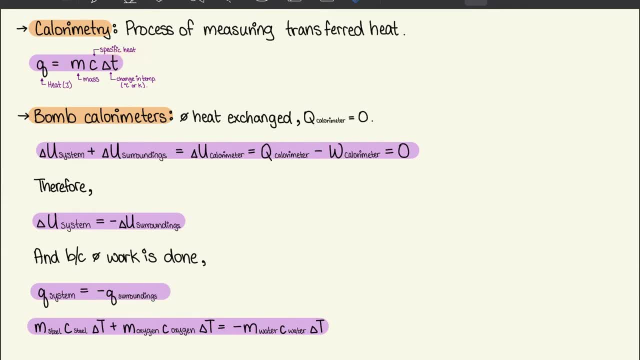 We have the mass for M, The C is a specific heat constant and the delta T is the change in temperature. Now this could be either in both Kelvin or degrees celsius. Moving on to bomb kilometres, There is no heat exchange, so the Q value is equal to zero. 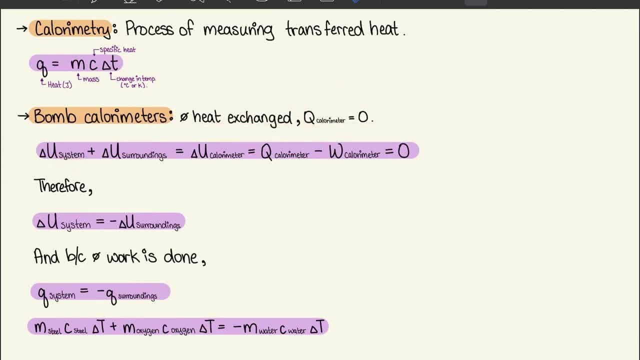 So we have the equation here. We have the delta U of the system plus the delta U of the surrounding, which would become delta U of the calorimetry is equal to Q. calorimetry minus W kilometre, which is equal to zero. 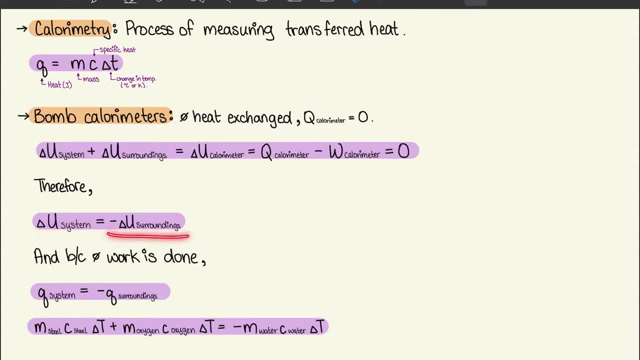 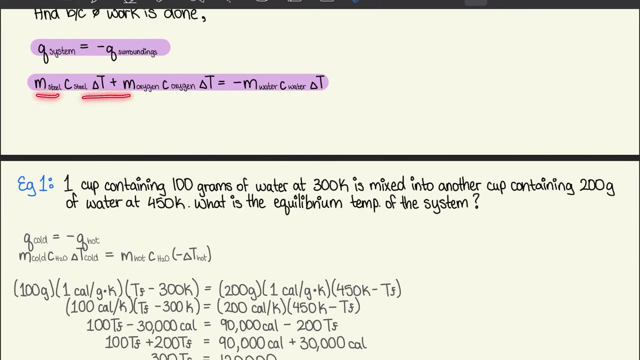 If we were to simplify this, it would become: delta U system is equals to quarter to negative Delta U surroundings and because no work is done, we come to Q system is equal to negative Q surroundings and we can further expand this equation with the Q is equal to MCAT equation for both sides. just pause. 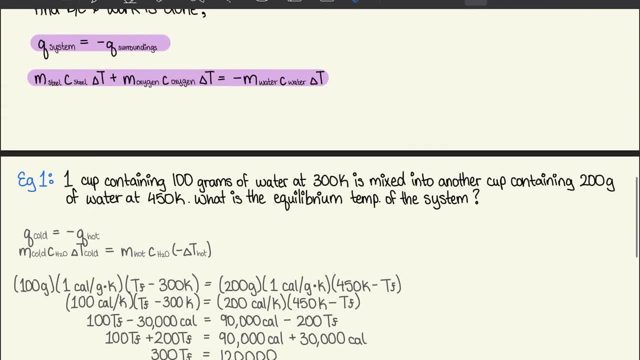 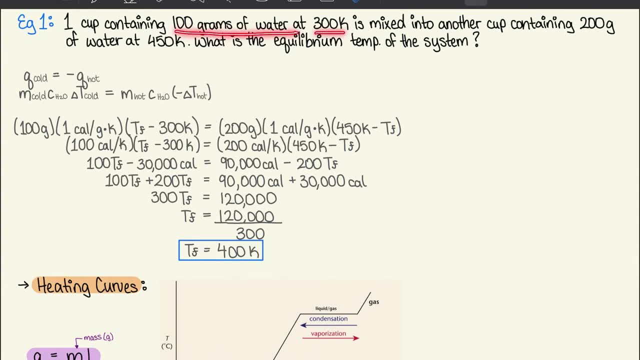 the video. have a look, see if you understand this. once you do, we have an example right here. so the example is: 1 cup containing 100 grams of water at 300 Kelvin is mixed into another cup containing 200 grams of water at 450 Kelvin. what is the equilibrium temperature of the system? so we're gonna 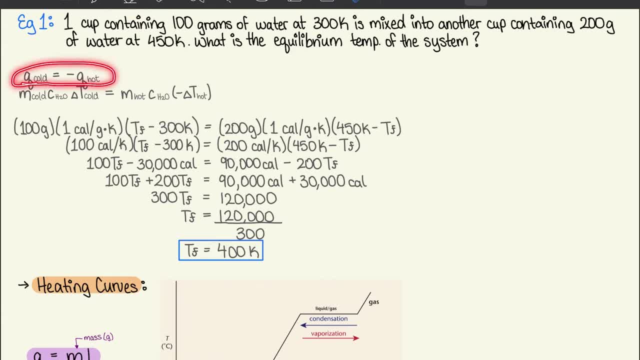 write: Q cold is equal to minus Q hot and that's for the different temperatures. so we're going to expand that into M cold, C for water and Delta T cold for the colder temperature, and then M C, H 2 O and negative Delta T for hot- we're going to expand- and for mass cold 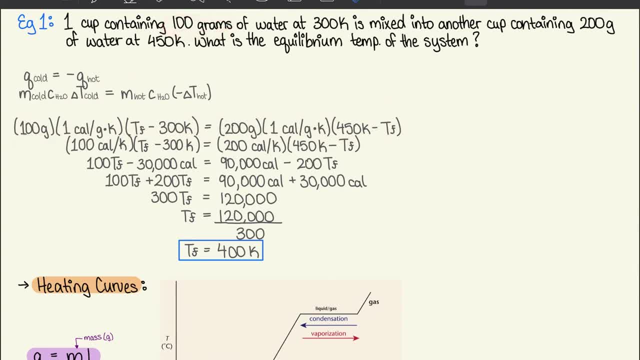 we have 100 grams. that's already given in the equation. we're going to use our specific heat constant for water, which is 1 Cal per grams times Kelvin, and because the constant has a Kelvin, we're going to make sure that our temperatures are in Kelvin as well when we input them in. so we have our TF minus 300 Kelvin. 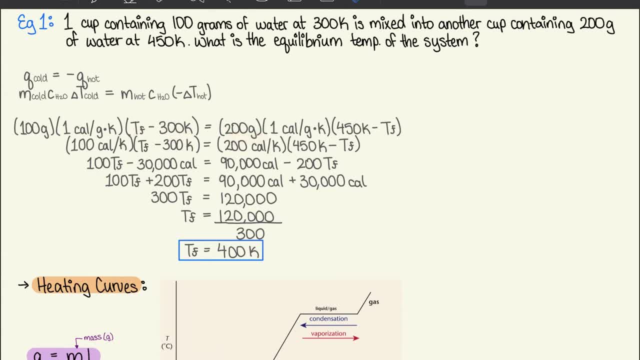 is equal to 200 grams of the mass of the hot substance of water and we have this same specific heat capacity and then we have 450 Kelvin minus TF. we're going to simplify all of this through where our TF is equal to 400 Kelvin, and that's our. 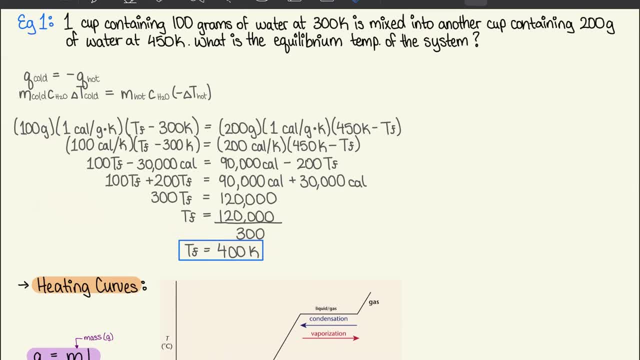 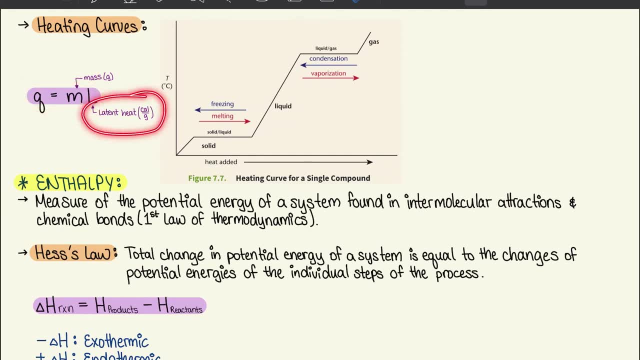 answer. so we're going to move forward to the heating curves where Q is equal to ML grams and L is latent heat, where it's cal over grams, and that's the graph for that. So pause the video, make sure you understand this graph and how it correlates with the equation, and once we're, 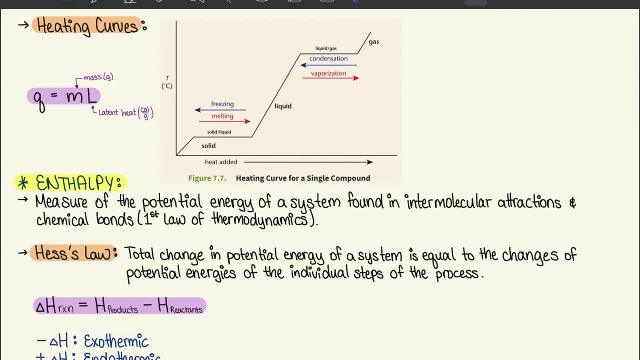 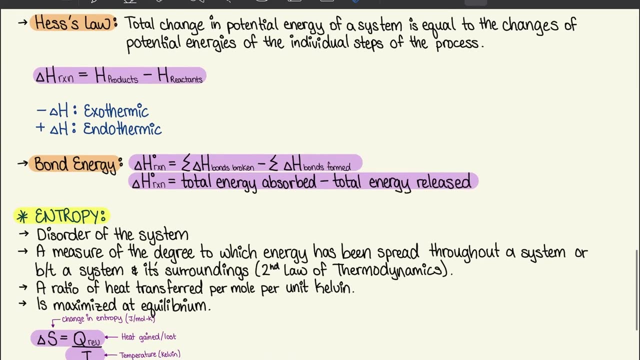 all good, we're going to move forward to 7.4, where we talk about enthalpy. Now, enthalpy is the measure of potential energy of a system found in intermolecular attractions and chemical bonds, and that's the first law of thermodynamics that we talked about before. So for Hess's law, the 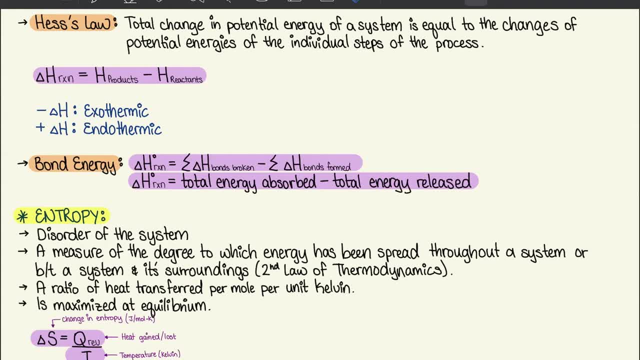 total change in potential energy of a system is equal to the changes of potential energies of the individual steps of the process, and we show this by the delta H equation here. So delta H reaction is equal to H products minus H reactants. Now if we have a negative delta H value, we know that. 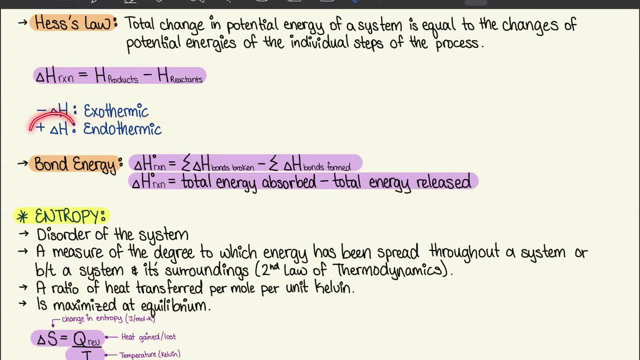 it's going to be an exothermic reaction. However, if we have a positive delta H value at the end, we know that this will be an endothermic reaction. So to calculate bond energy, we put delta H reaction is equal to the sum of the delta H bonds broken and the sum of 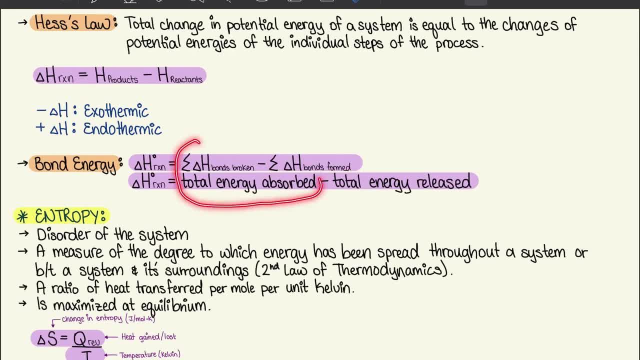 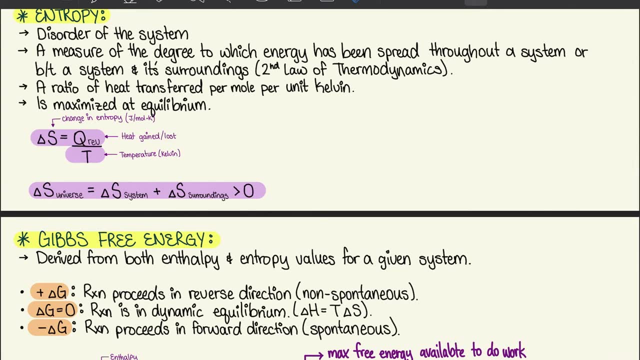 delta H bonds formed. So we can simplify this as total energy absorbed minus total energy released, Moving on to 7.5,. we talk about the entropy. so that's the disorder of the system. Another way to say that is the measure of the degree to which 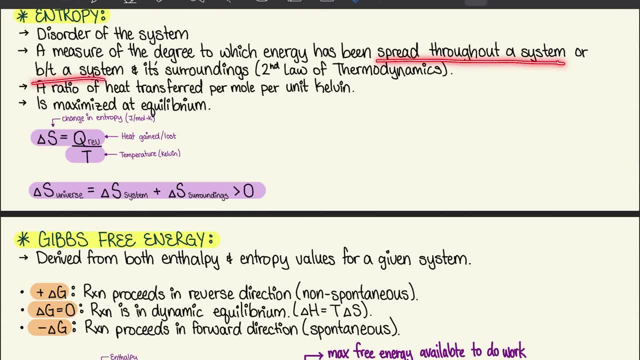 energy has been spread throughout a system or between a system and its surroundings, and that creates our second law of thermodynamics: A ratio of heat transferred per mole per unit Kelvin and is maximized at equilibrium. So this is the equation that we have where entropy is. 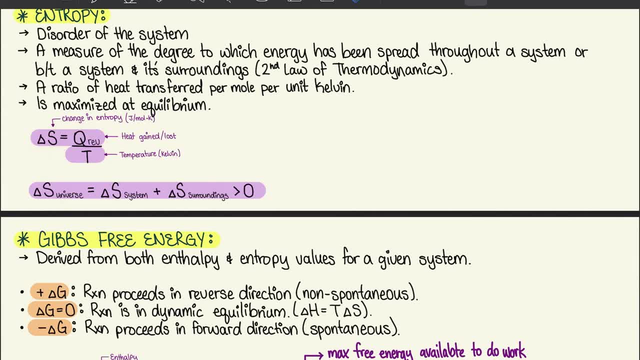 represented by delta S. So that's the change in entropy, and once again the units are equal to delta S of the system plus the delta S of the surrounding, which has to be greater than zero. And next we're going to move on to chapter 7.6, where we talk about Gibbs, free energy. 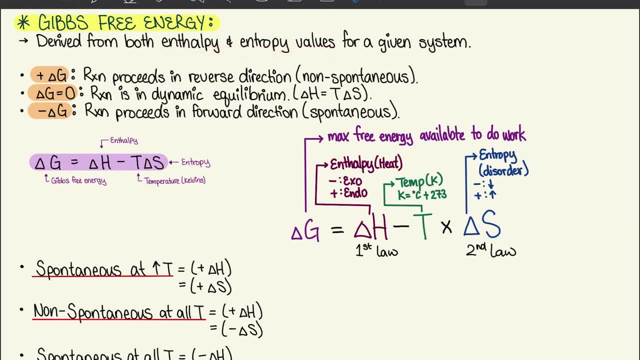 So it's derived from both enthalpy and entropy values. So we have a given system. Like we said before, when we have a positive delta G, we know that it's non-spontaneous and it's going to proceed in the reverse direction. 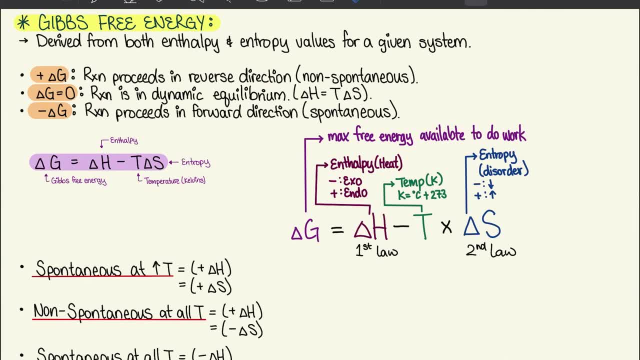 A delta G value that's equal to zero will be in equilibrium and we can write that, as delta H is equal to T delta S, where delta H is enthalpy, which is the heat, is equal to temperature times entropy, which is delta S, And negative delta G is equal to T delta S, which is the heat. 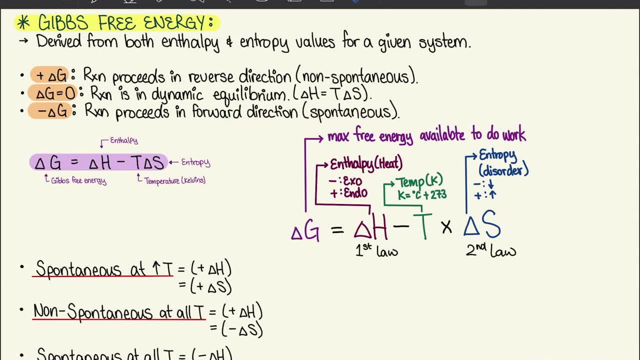 and the energy value proceeds in the forward direction and is spontaneous. So overall we can write that delta G, which is Gibbs free energy, is equal to enthalpy minus temperature, times, entropy. And on the side here we have if delta H is positive or negative. 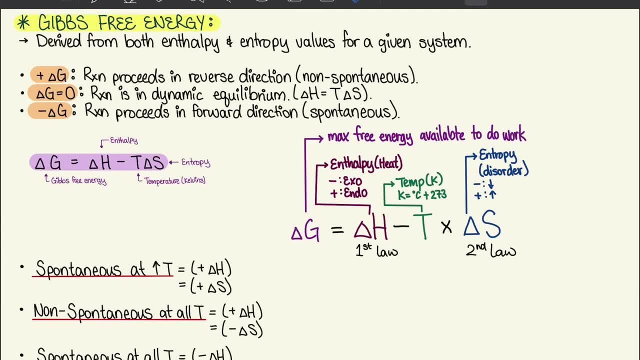 it's either exo or endo, and temperature is in Kelvin, where it's degrees Celsius plus 273 to get our Kelvin value, And entropy, which is T delta S, is equal to T delta S, which is T delta S. 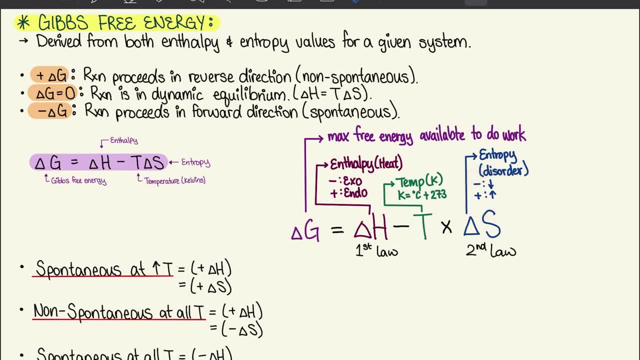 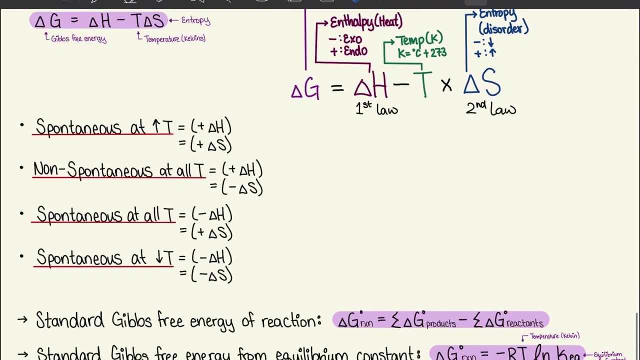 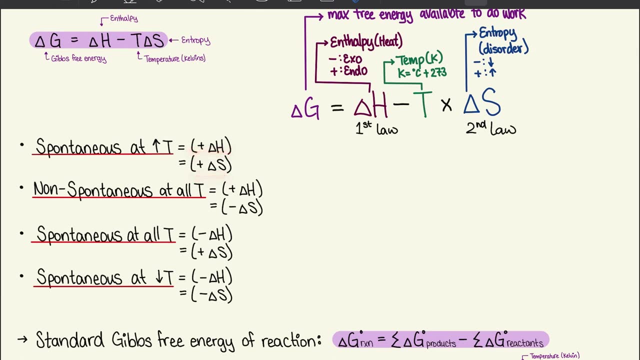 which is the disorder. If it's negative S, it will decrease and positive delta S will increase the disorder. So this is spontaneous at higher temperatures, where we have a positive enthalpy value and a positive entropy value. For non-spontaneous, at all temperatures, we have a. 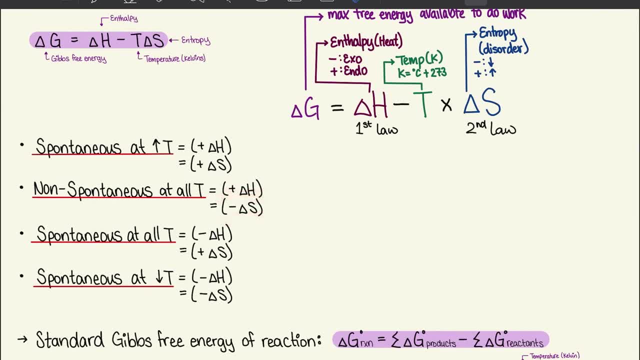 positive enthalpy value and a negative entropy value, And spontaneous at all temperatures. it's negative enthalpy And positive entropy And spontaneous. at lower temperatures we have a negative entropy and negative enthalpy as well. So standard Gibbs, free energy of a reaction, we have the equation. 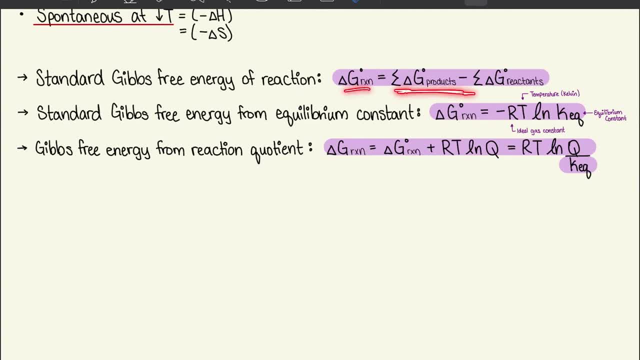 delta G reaction is equal to the sum of the delta G of products minus the sum of delta G of the reactants And the standard Gibbs free energy. of equilibrium constant we have delta G reaction is equal to negative RT, ln, Keq, Where R is the ideal gas constant, T is the temperature in Kelvin and Keq is the equilibrium. 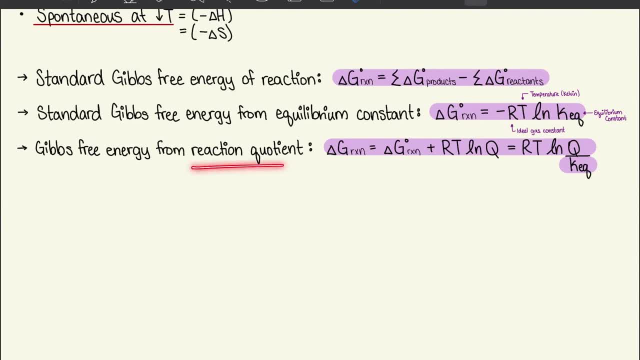 constant And Gibbs free energy from reaction. Quinton is the same thing, except we go. delta G reaction is equal to the standard Gibbs free energy plus RT. ln, Keq Instead of Keq. we have the Quinton in this equation And we can simplify that further where RT is.